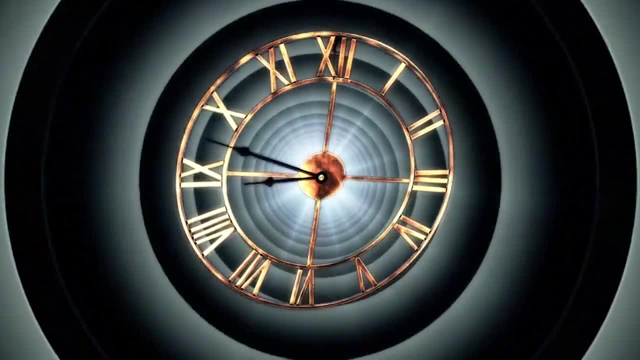 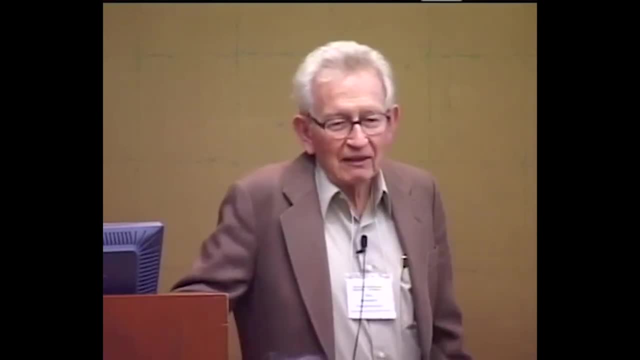 Anderson in his super non-youthful prime, giving a lecture on something I am thoroughly not aware of, because I just really wanted a video of him. Philip Warren Anderson is a particle physicist who worked in the field of symmetry, breaking particle physics. This allowed other physicists 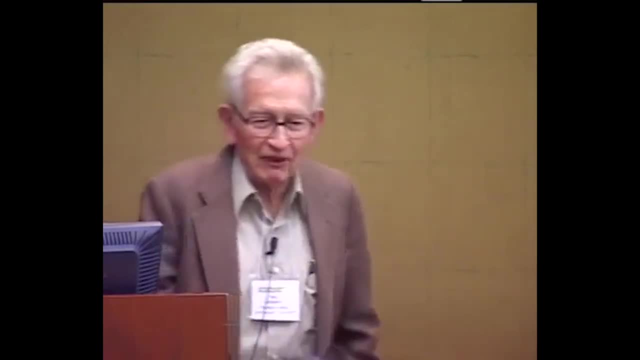 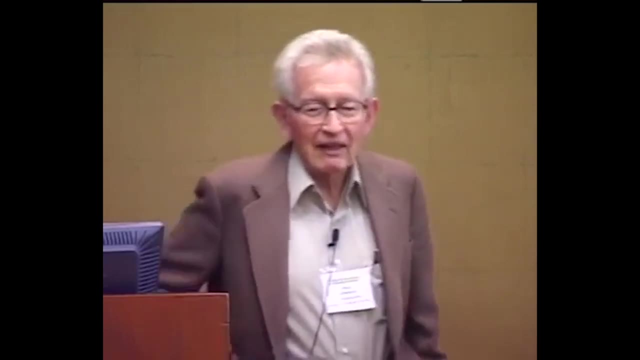 to come up with the proposition of spontaneous symmetry breaking when referring to the Higgs field and its interactions with elementary particles. He was employed by Bell Labs, working on a variety of problems revolving condensed matter physics. The main takeaway is that he helped in furthering the ambition towards the Higgs mechanism. 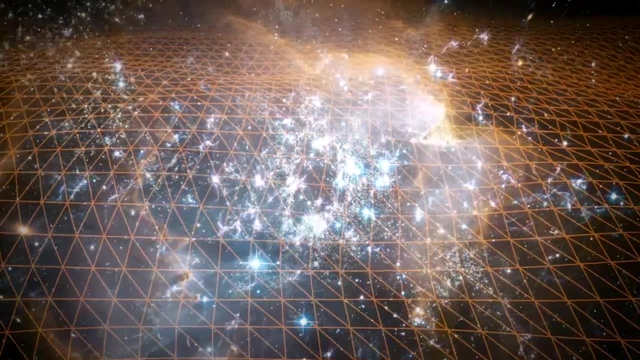 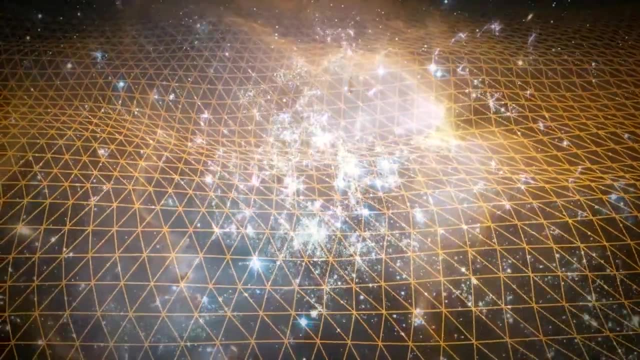 Now I know what you're thinking: he is rambling on about elementary particle physics and standard models. but what is the Higgs mechanism itself? Well, let's first begin with the Higgs field. But let me first ramble a little more and introduce Robert Bout, François Englert. 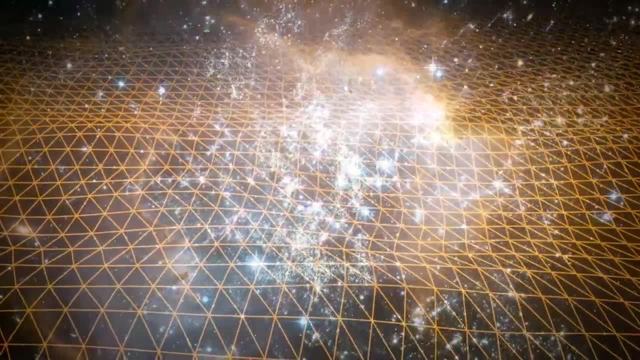 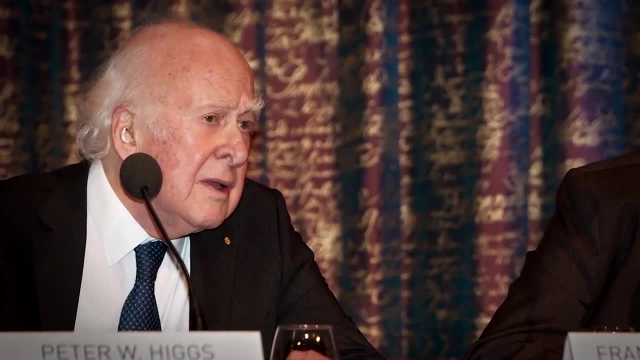 and Peter Higgs. By the way, most clips really emphasize Peter Higgs, so here is him until I finish this paragraph. These three physicists were able to surmise the idea of a permeating mass-giving field, which was first called the Brout-Englert-Higgs mechanism. This led to the 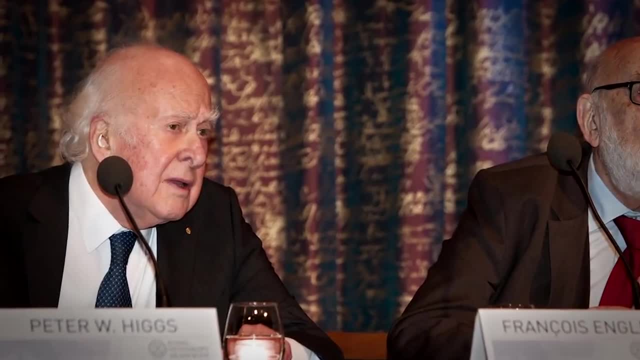 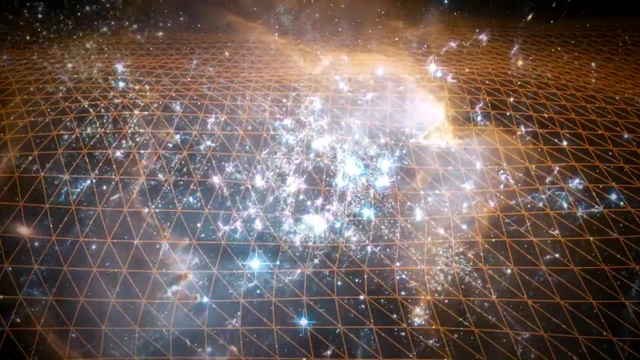 first theorization of a field of which particles interact with to obtain mass while maintaining the nice structure of their original interactions. Now back to the Higgs field itself. It is theorized that elementary particles that make up matter interact with the field in varying 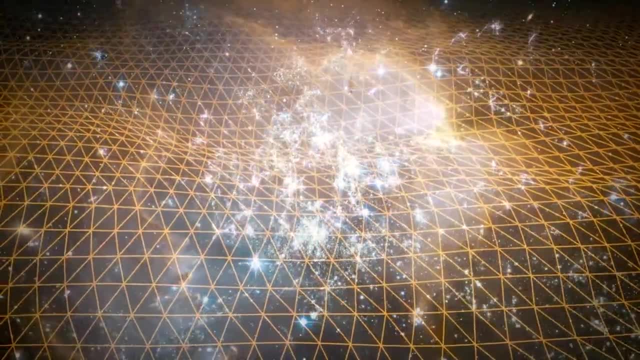 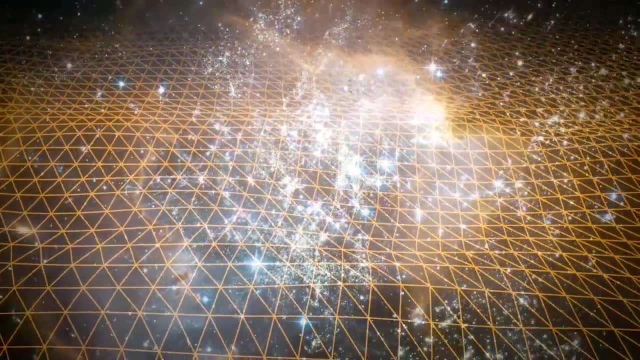 ways. Thus, this particle interaction with the Higgs field gives them their mass property. It is also stated that the more a particle interacts with the field, the more mass that particle has. Therefore, mass is solely dependent on the particle's interaction with the Higgs field. 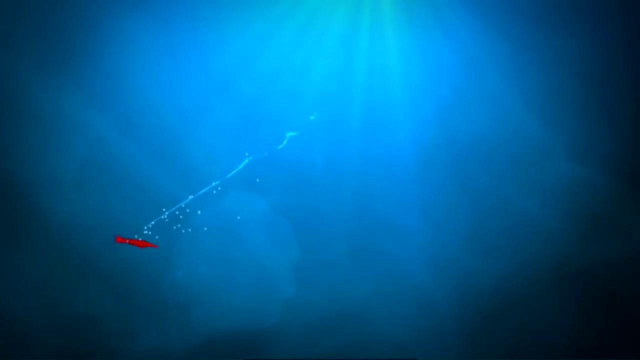 Consider a small fish moving about in water. The shape of the fish is pointed and so it is able to move very quick, interacting very minimally with the water's resistance. Now this cube has a flat surface on all of its sides and intuitively it interacts much. 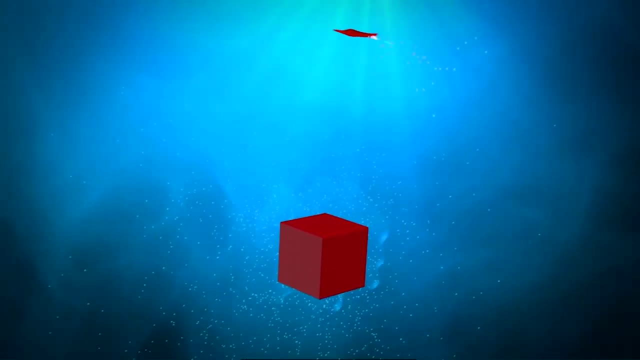 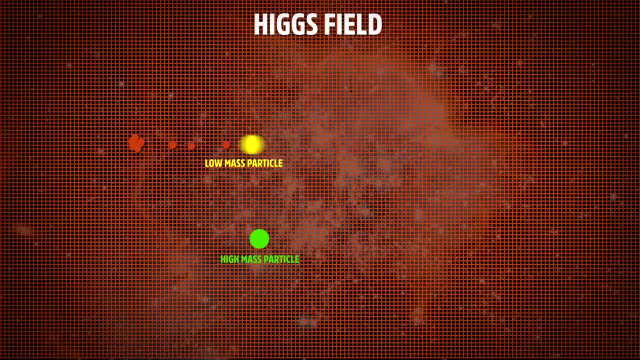 more with the water's resistance, therefore causing it to move slower than the pointed fish. We can compare this with the Higgs field, where particles that interact less with the Higgs field have a smaller mass than particles that interact more with the Higgs field, giving them a larger 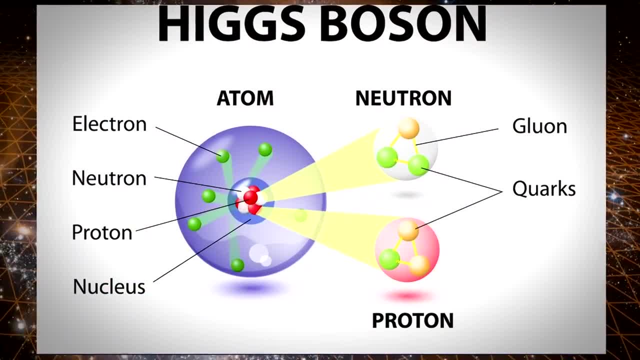 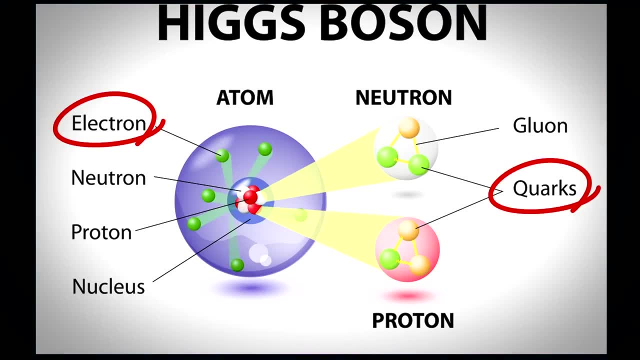 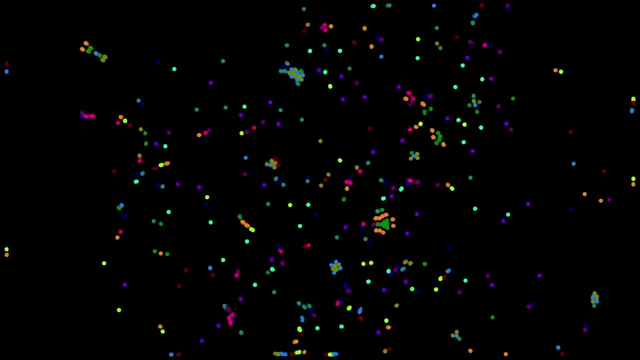 mass. To further elaborate on the revolutionary idea of the Higgs field, we should also note that the Higgs field is used as a way of explaining the mass given to particles such as electrons and quarks. Now that we have taken a look at the Higgs field, let's begin to dive into the nitty-gritty. 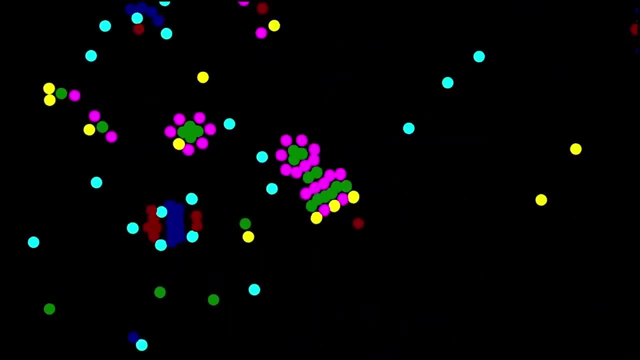 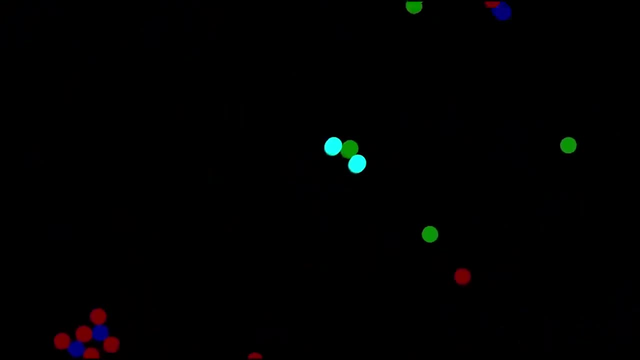 And the nitty-gritty will be the actual particle interactions. You may wonder: what exactly do the particles interact with in the Higgs field? Well, judging by the video playback that is playing over top of my voice, I am hoping that you would guess. yes, that's right. particles, The Higgs. 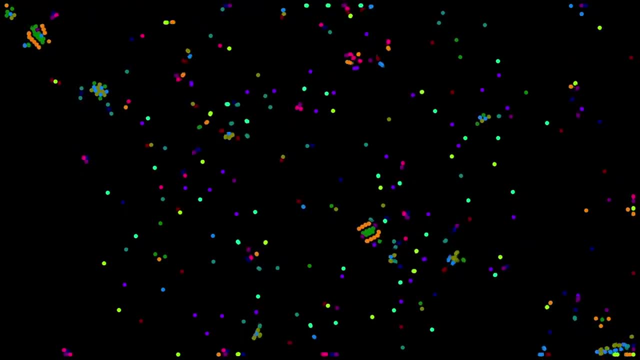 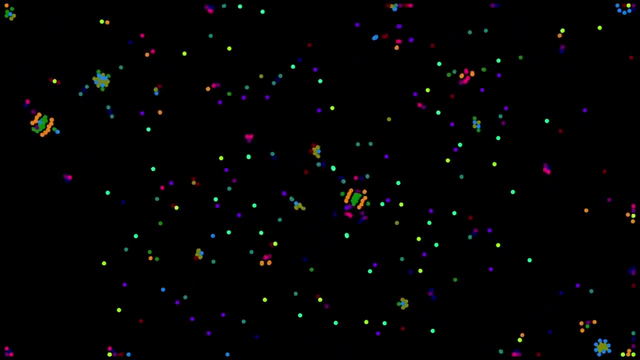 field is made up of particles known as the Higgs boson. More specifically, it is a certain density of these particles that permeate the so-called field. I say so-called because it is quite literally a field of particles. The Higgs field is made up of particles known as the Higgs boson. 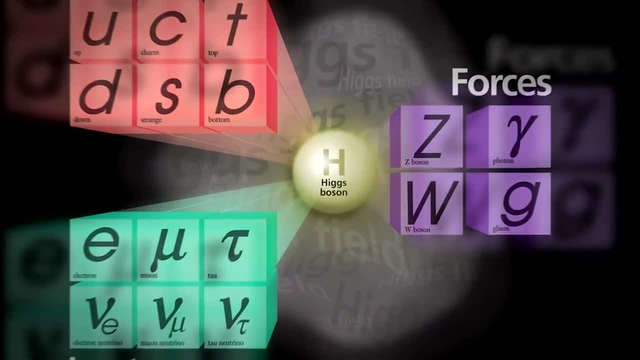 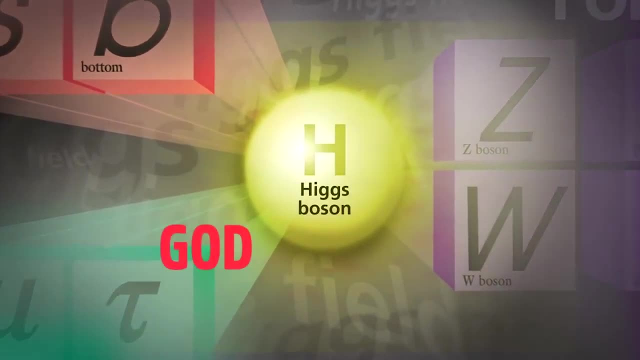 To jog your memory a bit, you may have heard of popular science articles write about the revolutionary God particle. Well, I guess you can think of it how you will, but it is quite a fundamental particle in our universe and without it we would be massless. I don't even 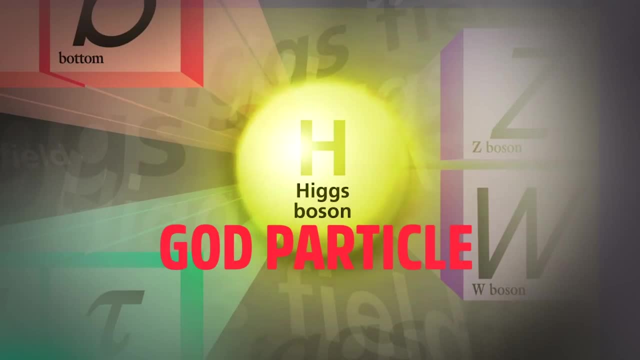 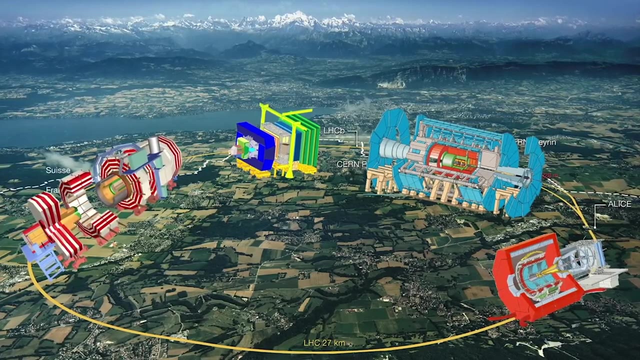 know what's moving through space at the speed of light. Now, as of 2012 and 2013,, the Higgs boson has been conclusively- based on probabilistic and statistic means which are beyond our level of understanding, been confirmed to have been found. These experiments were conducted at CERN's 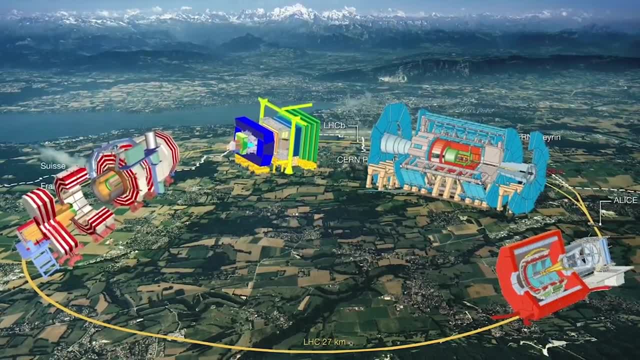 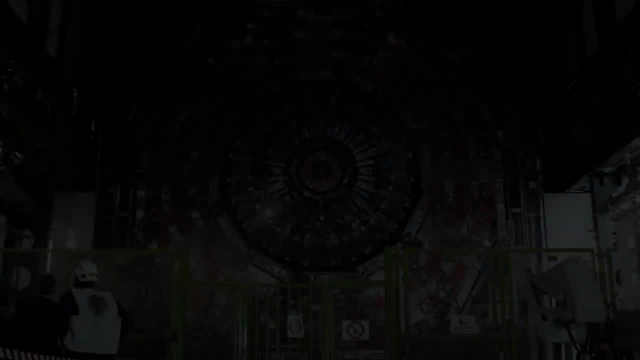 Large Hadron Collider and the energy levels of the Higgs boson were detected through the general purpose detectors ATLAS and CMS. Now, I didn't really mean to make you a guest by saying the probability and statistics regarding particle physics is way beyond our. 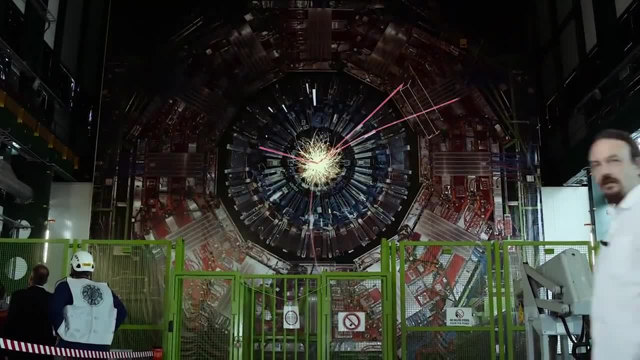 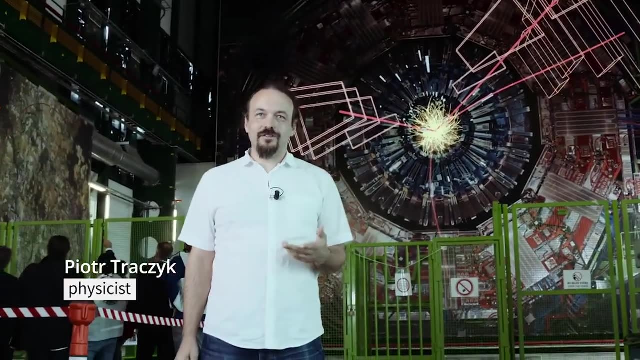 understanding, but it is quite complex and it should be thought of as a tremendous feat in the field of particle physics. I won't delve too far into the maths, but you should note that when they are quantifying the findings for certain particles, it's based on standard deviations using data. 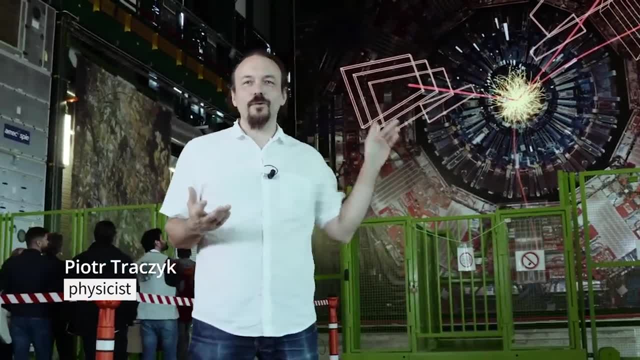 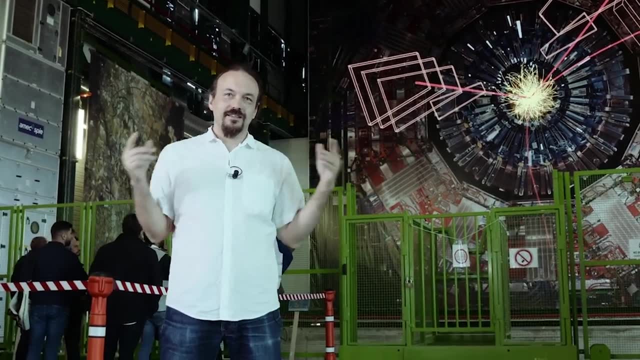 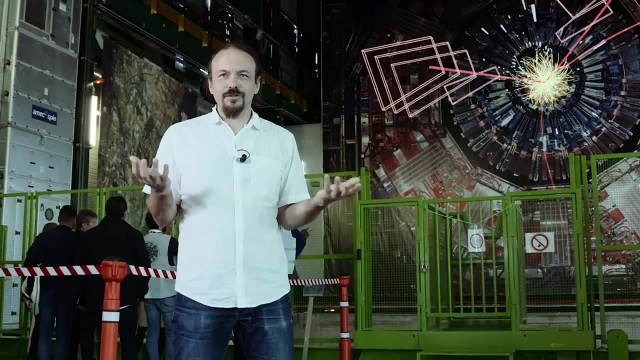 lists and CMS. These are not your typical standard deviation calculations, as there are a lot more in-depth analysis conducted by researchers Now regarding the computational probabilities. physicists base these p-values on the chances of not finding the particle. In the case of the Higgs boson, it is said that the probability based on the researchers' analysis